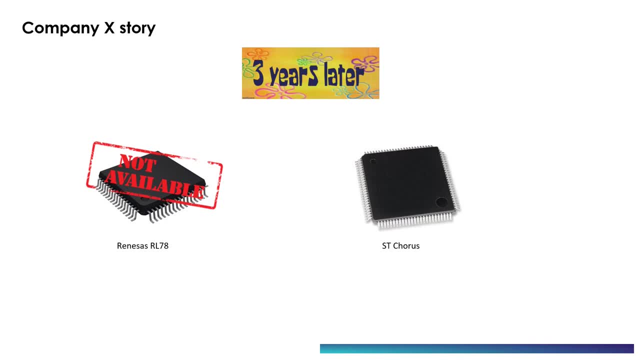 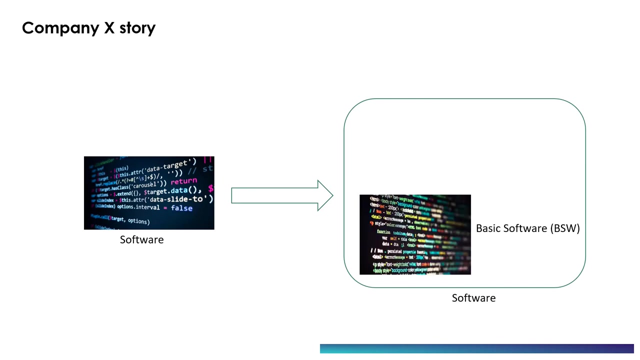 different architecture than the previous one. The previous software was so much dependent on the controller specifics that they cannot reuse it anymore. Hence this time, company X decides to write the software in two parts: BSW layer, which controls the hardware and provides system functionalities, and ASW layer, where the application for BCM is written. 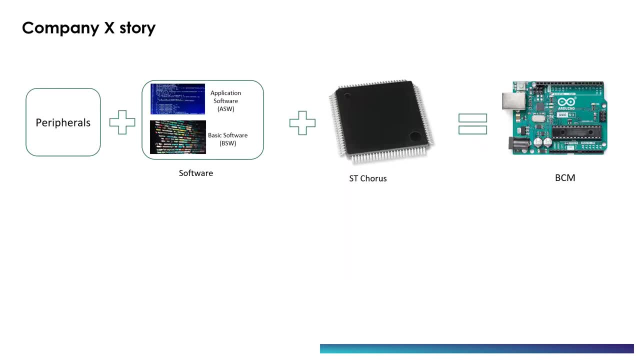 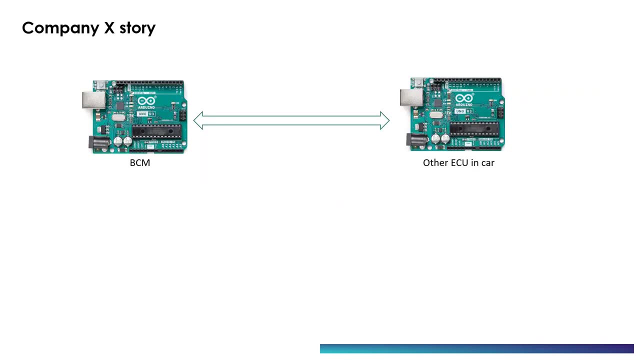 Okay Now, when they test the software in a standalone mode, it works, But when they test the software with other modules in the car, it doesn't work anymore due to some compatibility issues. So basically, this shows how important a hardware and software portability is. A small change. 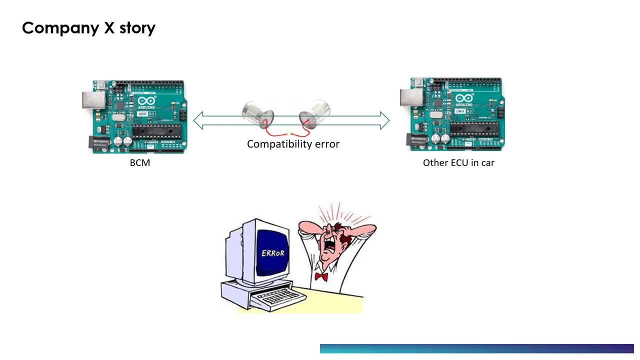 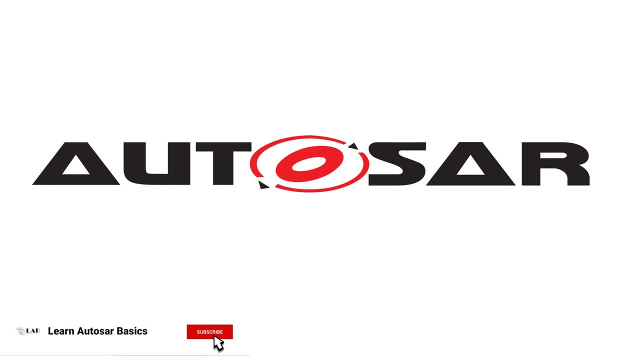 in architecture requires whole system to be redesigned. This rework and lack of coordination between tier 1 suppliers and OEMs in 2003 is a major problem. In the early 2000s, OEMs gave birth to a standard called Automotive Open System Architecture. 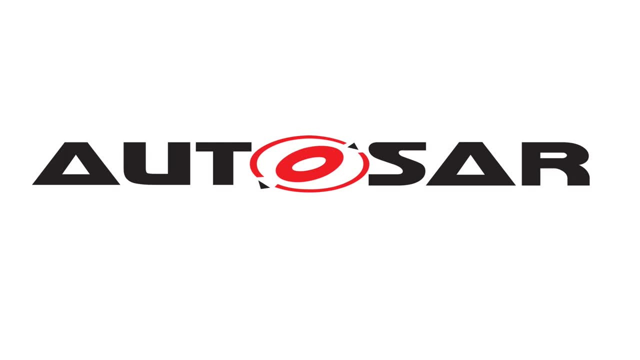 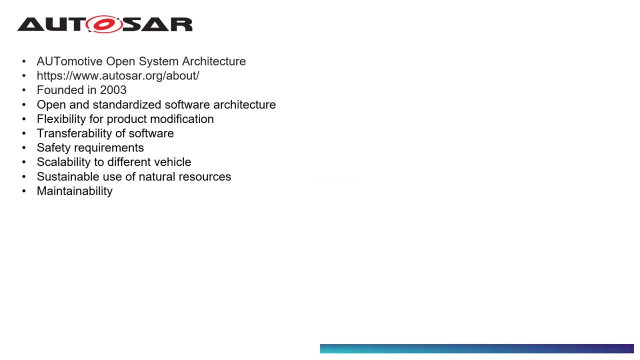 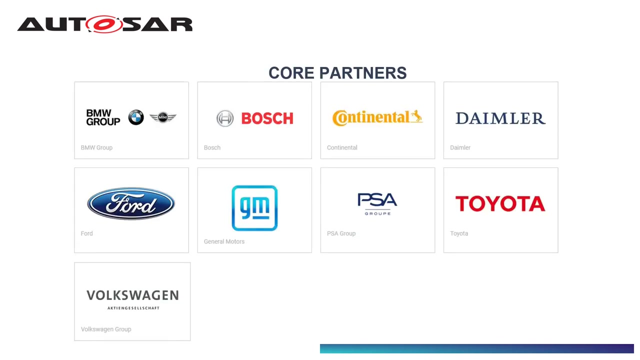 or very well known as AUTOSAR. The motivation behind AUTOSAR was to increase the flexibility for product modification and to leverage the scalability of solutions across ECUs. It also motivated reliability and quality of the software and safety requirements. More details about AUTOSAR can be found on AUTOSARorg website. Here is a list of core partners in: 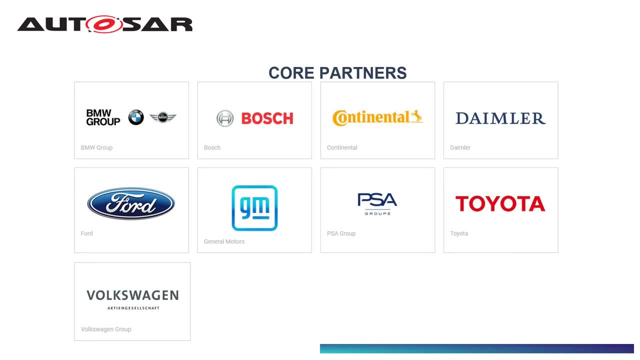 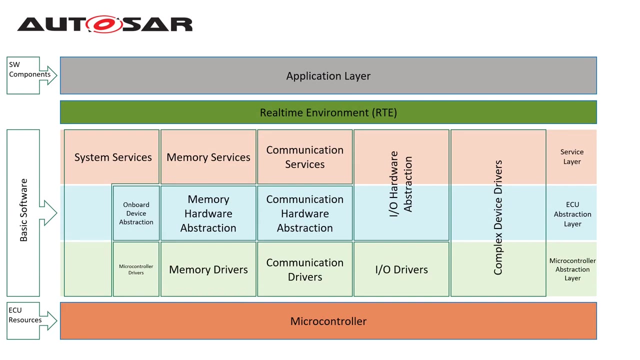 AUTOSAR consortium. We have BMW, Bosch, Continental, Daimler, Ford, General Motors, PSA Group, Toyota and Volkswagen. AUTOSAR follows a three-layer architecture. We have application layer, real-time environment layer, or RTE in short, basic software layer, or BSW in short Software, which is a combination. 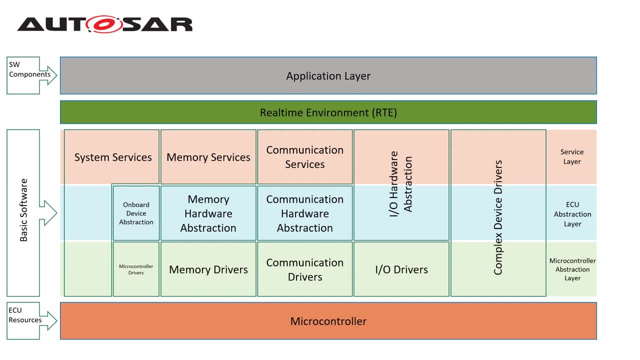 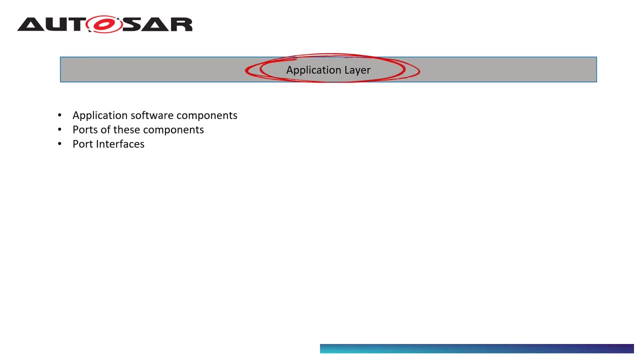 of these layers run over a microcontroller. Now let's try to understand these layers one by one. First we have application layer. This layer includes various application-specific components which are designed to execute specific set of tasks. Software components are nothing. 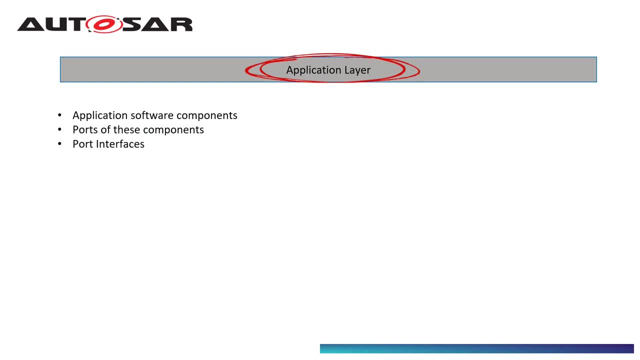 but the simplest form of application. Application layer is made up of three parts: Application, software components, ports of these components and port interfaces. Next layer is RTE. It is a middleware layer between application and basic software layer. It provides communication channel between software components and BSW using ports and 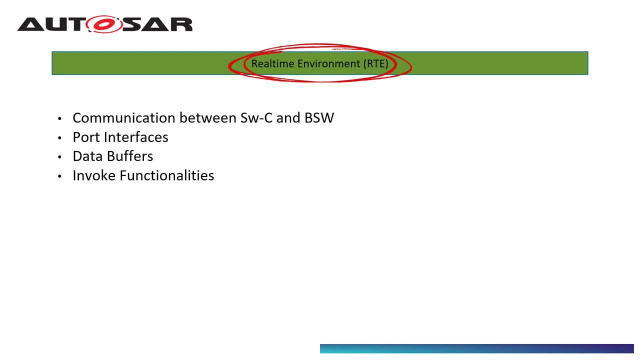 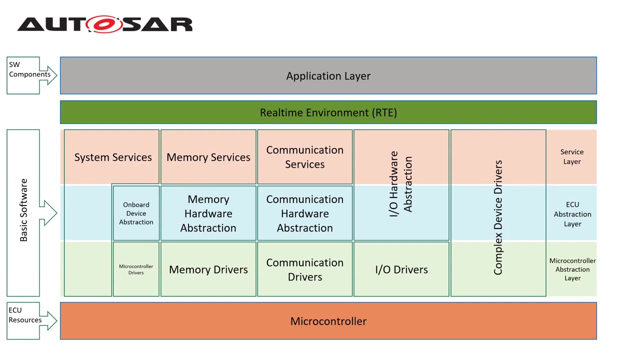 port interfaces. These ports exchanges data using RTE buffers and invokes BSW functionalities. Another interesting fact about RTE is that the software architecture about RTE changes from layer to component style. Lowest software layer is BSW layer. It is a standardized software that can provide services to autosar software components. It 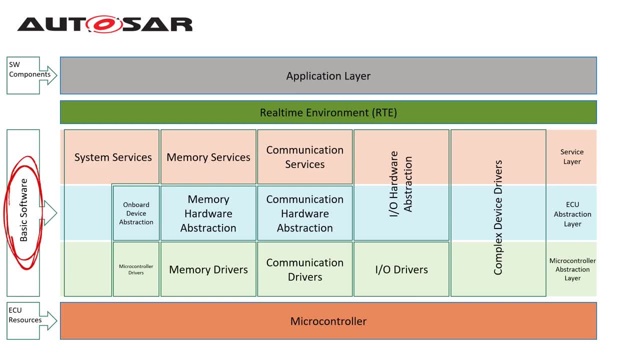 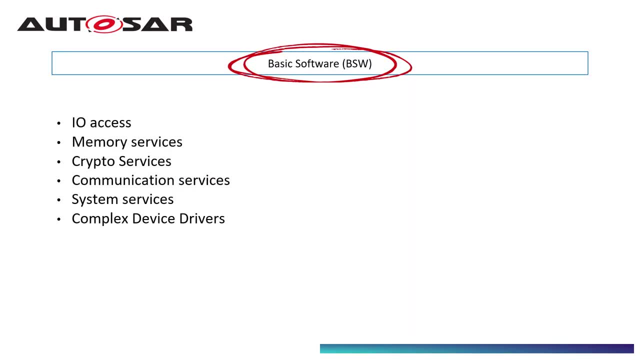 is also used to run the functional part of the software. BSW includes standardized and ECU-specific components. BSW layer provides the following services: Input-output: This provides access to sensors, actuators and various peripherals. Then we have memory: This provides access to internal and external memory. Then we have crypto: This provides 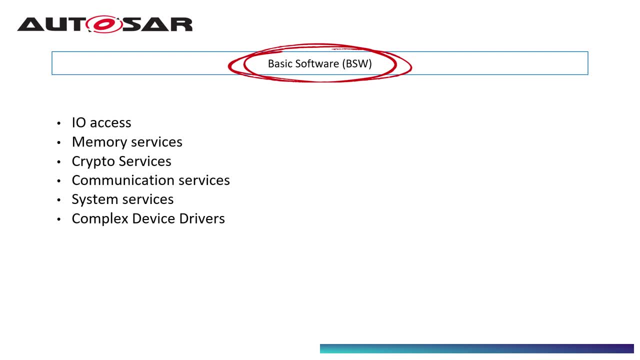 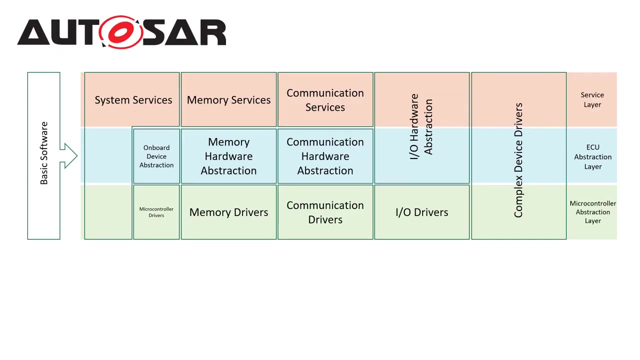 cryptographic primitives. Then we have communication. This provides various communication protocols for on-board and off-board communication. Then we have system. This provides ECU-specific services and library functions. BSW layer is further subdivided into three horizontal layers. We have service layer, ECU abstraction layer, microcontroller abstraction layer or 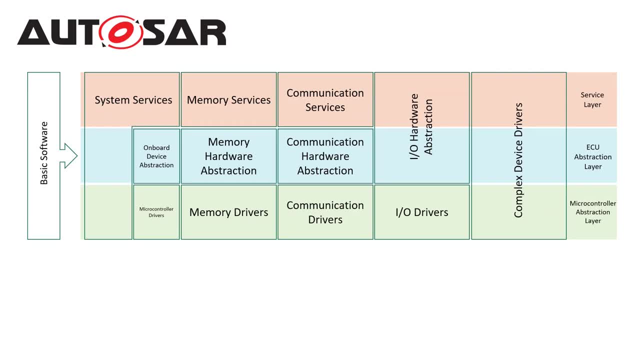 MCAL. Let's have a look at them one by one. First is service layer. This is the topmost layer of BSW. It provides interfaces to the application which are independent of microcontroller and ECU hardware. Then we have ECU abstraction. 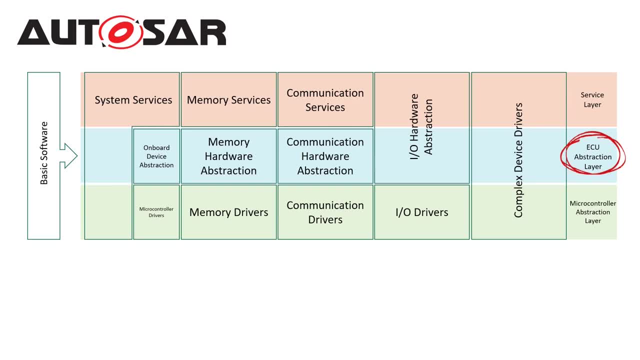 layer. This layer offers uniform access to all the functionalities of ECU, such as communication, memory or IO, regardless of whether these functionalities are part of controller or are implemented by peripheral components. It also offers API to interface with the microcontroller device drivers. 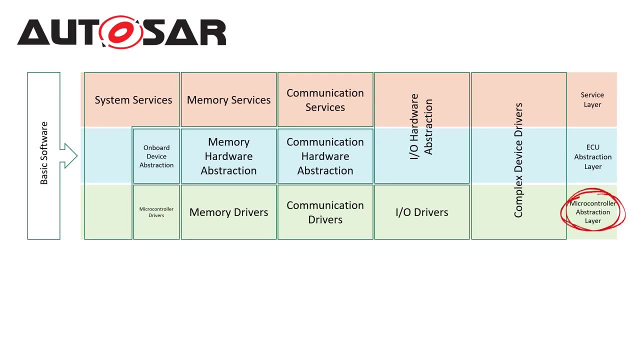 The lowest BSW layer is MCAL or microcontroller abstraction layer. It is access route to communicate with the hardware. It contains internal drivers which are software modules which have direct access to the microcontroller and internal peripherals. This layer provides microcontroller independent values for BSW components. 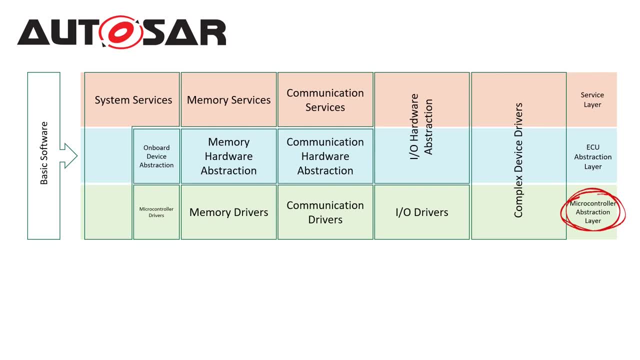 This is the corner of MCAL and ES herzlichTalks. long host network regulations, features in ecosystem installation area, bio-controller, temporal memory, computers and aircraft performance gains. İn campus things come into play, such as장이 Jest Приre pipes in DC or VR. guests can contact blockchain system services In-边 SDW can be seen to an external 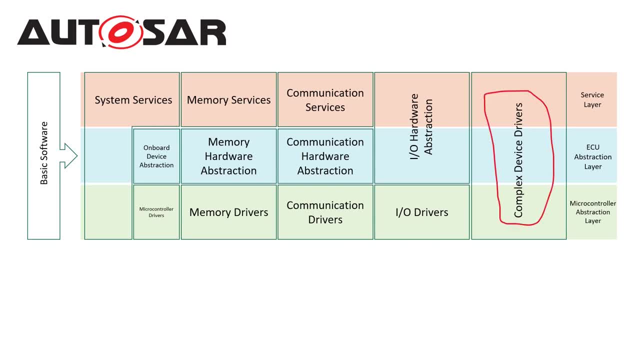 complex device driver layer, or CDD in BSW, which is not in a horizontal space but rather in a vertical space. This layer has special timing and functional requirements for dealing with complex sensors and actuators. CDD is used for handling complex functions that can't 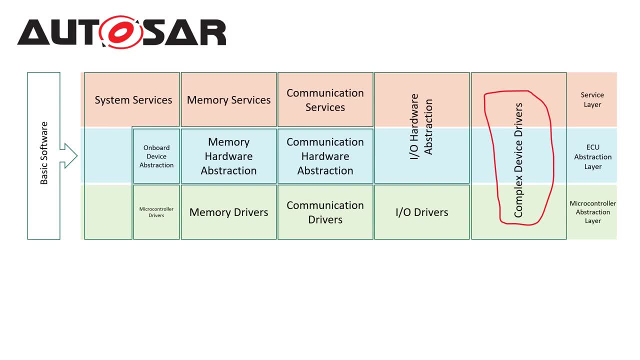 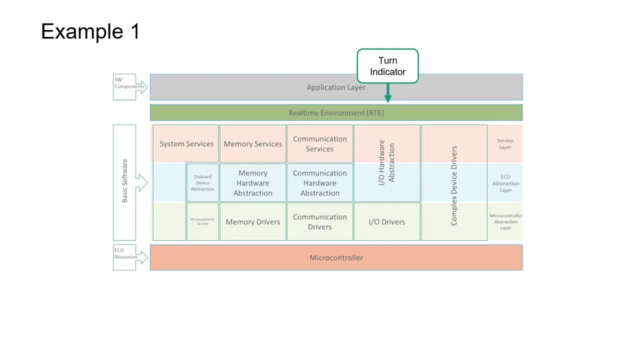 be found in any other BSW layer. It also has the ability to access the microcontroller directly. Okay, so now let's try to understand a simple working principle behind a turn indicator on and off mechanism using AUTOSAR compatible software. The first step is that a software component for turn indicator requests to turn. 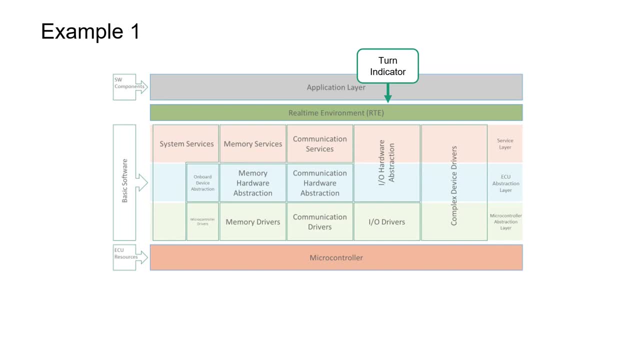 on the bulb. This request is routed through RTE to BSW responsible layer. In this case it is I-O hardware abstraction. This in turn switches on PWM signal to the signal on the output pin where the bulb is connected. Let's take another example. In this case, door control unit wants to broadcast the status. 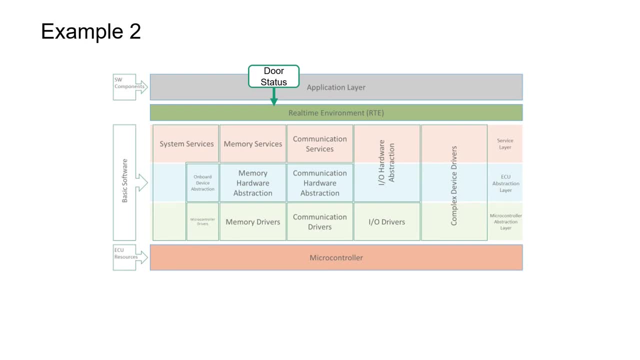 of door via CAN to other ECUs in the car First door. status software component in the application requests RTE to send a CAN signal. This request is routed to communication layer of BSW Communication service. layer routes the frame through CANIF to CAN driver. 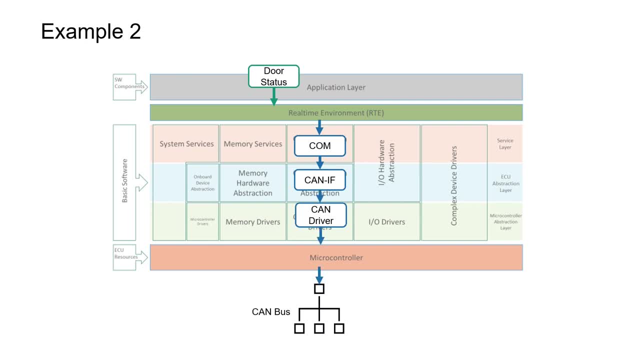 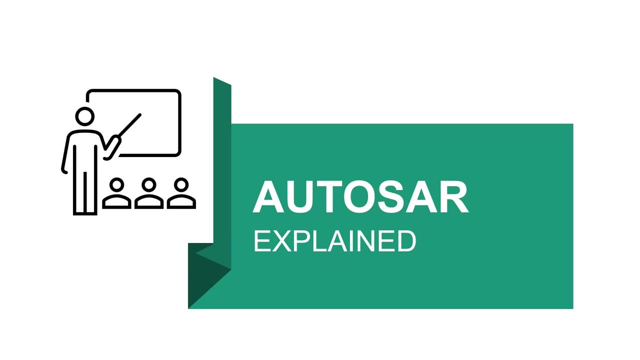 CAN driver helps writing the CAN frame into the hardware buffer, which in turn converts the buffer to electrical signal, which are then transmitted through the CAN bus to the other ECUs. I hope this video helped you to understand the basic principles behind AUTOSAR. If you. 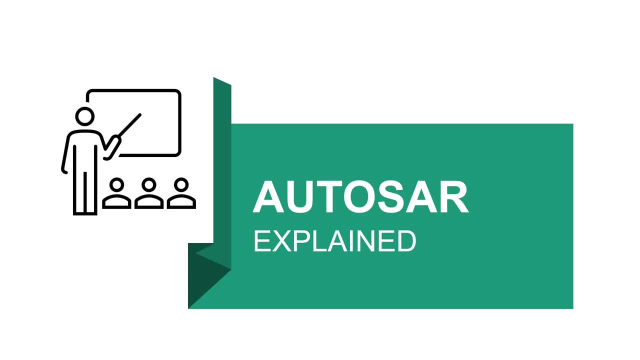 like the video. please don't forget to like, share and subscribe. Please let me know what other topics should we cover on this channel. Thank you and see you in the next video.